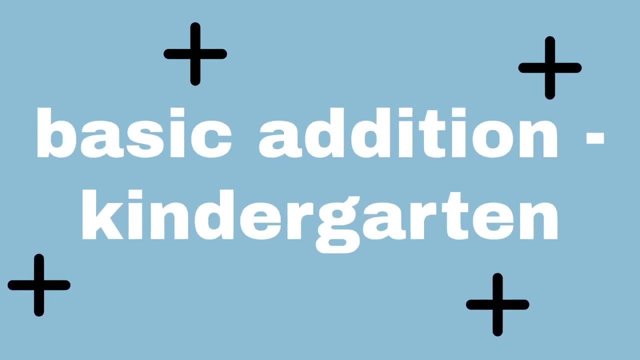 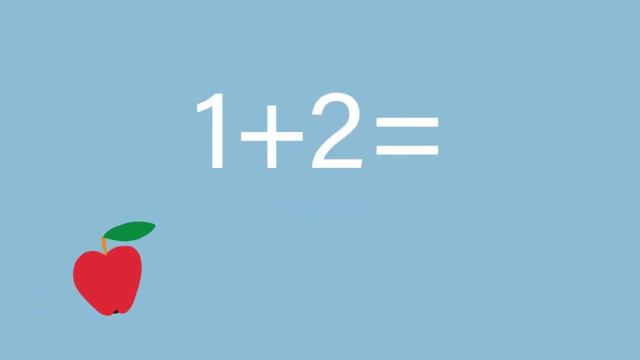 Hi, Let's learn basic addition. Are you ready? Let's go 1 plus 2.. There is 1 apple. Let's add 2 apples. Now we have 1 apple plus 2 more apples. This equals 3 apples. So 1 plus 2 equals 3, 2 plus 2.. There are 2 lollipops. Let's add 2. 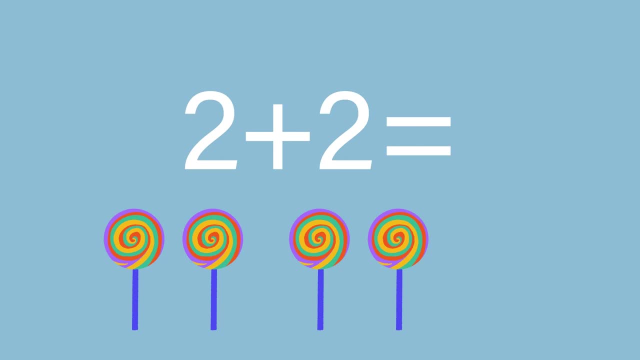 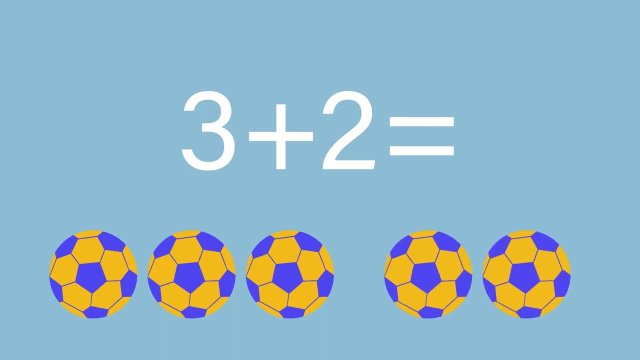 lollipops. Let's count the lollipops together: 1,, 2,, 3, and 4 lollipops. So 2 plus 2 equals 4.. 3 plus 2.. There are 3 balls. Let's add 2 balls. Now we have 3 balls plus 2 more balls. 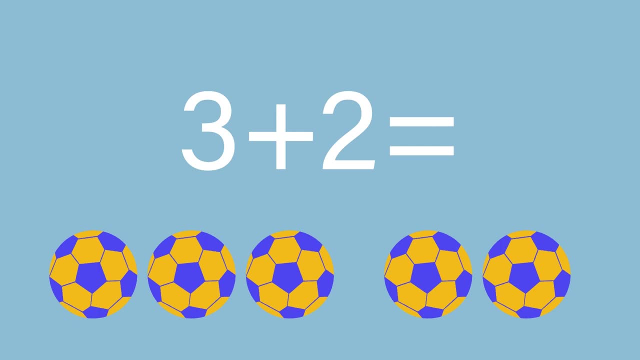 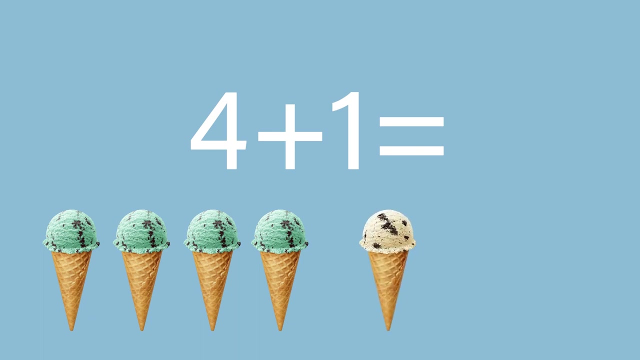 This equals 5 balls. So 3 plus 2 equals 5.. 4 plus 1.. There are 4 ice creams. Let's add 1 ice cream. Now we have 4 ice creams plus 1 more ice cream. 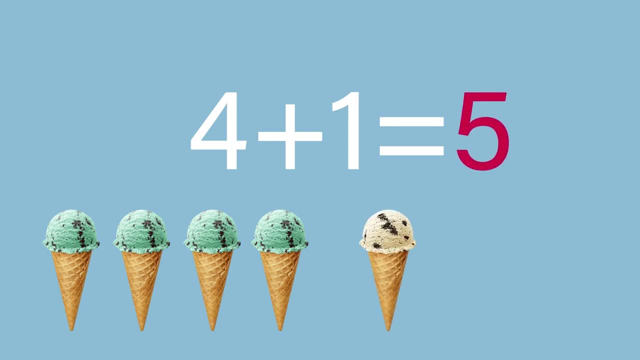 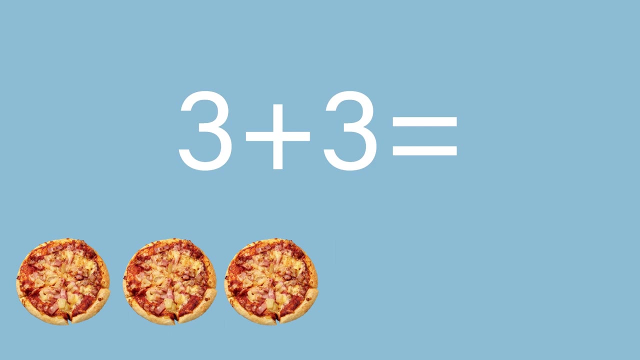 This equals 5 ice creams. 4 plus 1 equals 5.. 3 plus 3.. There are 3 pizzas. Let's add 3 more pizzas. Let's add 3 more pizzas. Now we have 3 pizzas. 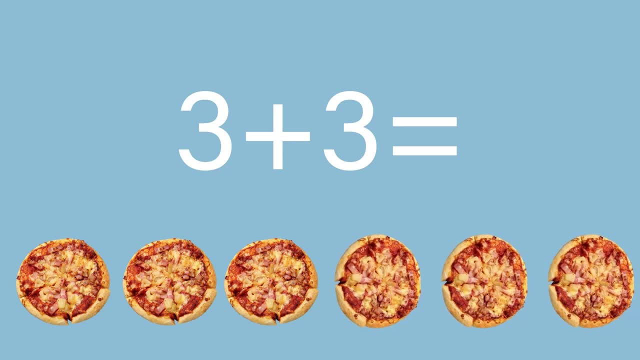 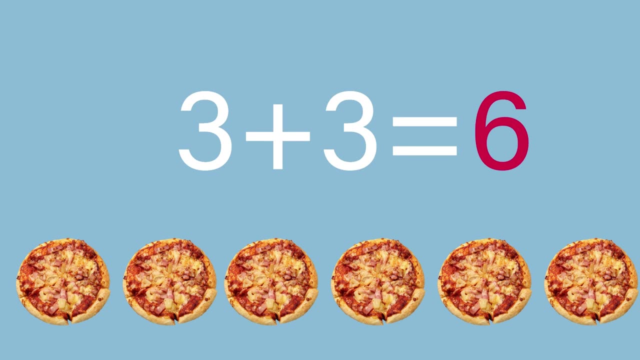 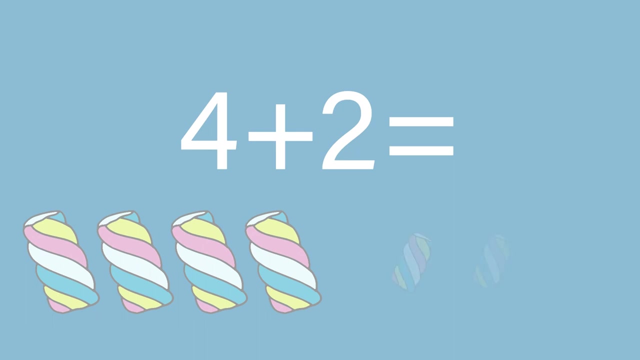 Plus 3 more pizzas. This equals 6 pizzas. So 3 plus 3 is 6.. 4 plus 2.. There are 4 marshmallows. Let's add 2 more marshmallows. Now we have 4 marshmallows plus 2 marshmallows. This equals 6 marshmallows. 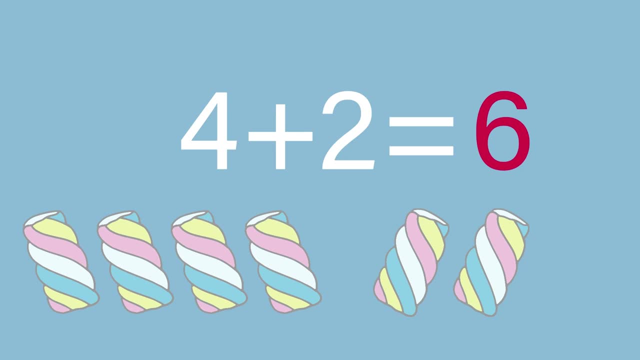 So 4 plus 2 equals 6.. So 4 plus 2 equals 6.. 5 plus 2. There are 5 pencils. Let's add 2 more. So 4 plus 2 equals 6.. 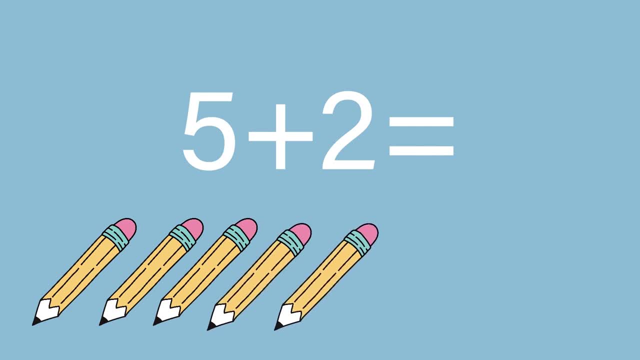 5 plus 2.. There are 5 pencils. Let's add 2 more. Now we have 5 pencils plus 2 pencils. Now we have 5 pencils plus 2 pencils. This equals 7 pencils. This equals 7 pencils.